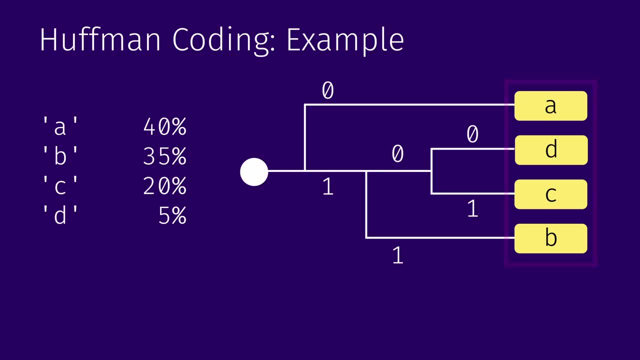 the leaves, and each leaf of the tree is a token. on this path, depending if we turn left to right, we can write zero or one, which will produce a prefix for this token. for example, if we try to encode a, we will go from the root left and we will immediately arrive at the leaf for a, so the 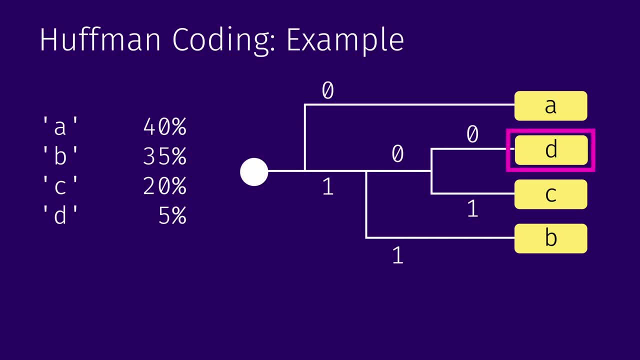 code for a is zero. if we will try to encode d, we will need to go from the root right, so it will be. then we need to turn left, that will be zero, and then we will need to turn left once more, which will be zero. so the prefix code for d will be one: zero, zero. we can repeat the same operations for b. 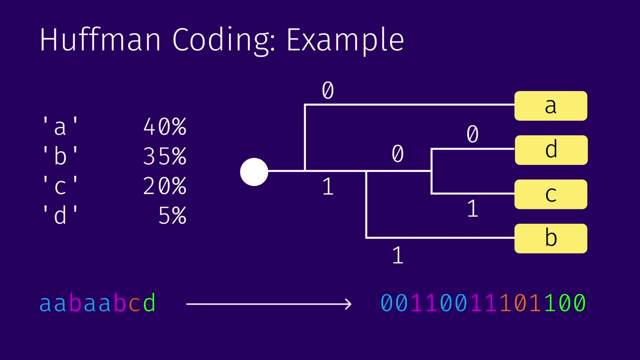 and c and if we take any sequence of those topics, we will get the same code tokens. we can now convert them to a corresponding code. if you want to decode it, we can just use the same tree to trace our paths to corresponding tokens. what is interesting here is that the size 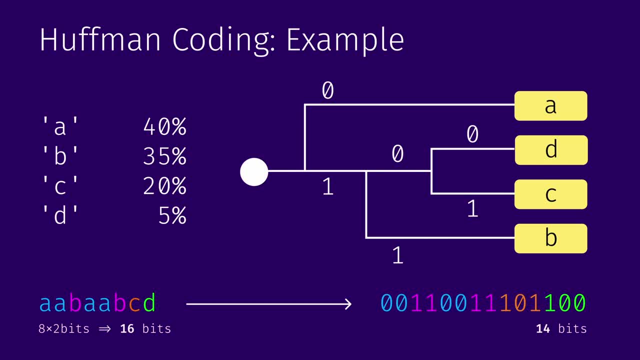 of this representation is less than the original representation. since we only have four options, it means that each token can be decoded in two bits. our string is eight tokens long, so to encode it we will need to use 16 bits, but if we use half man encoding we will only need 14 bits to encode. 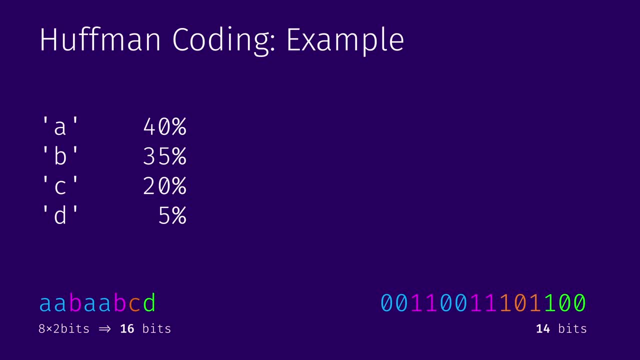 this. that's how compression is achieved. of course, tracing the tree is not the most optimal option most of the time, so normally you would try to create a hash map so you can map each token to its corresponding prefix, and you can create reverse hash map which will map prefixes to 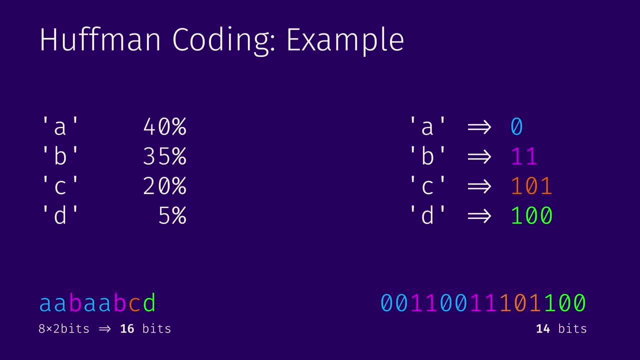 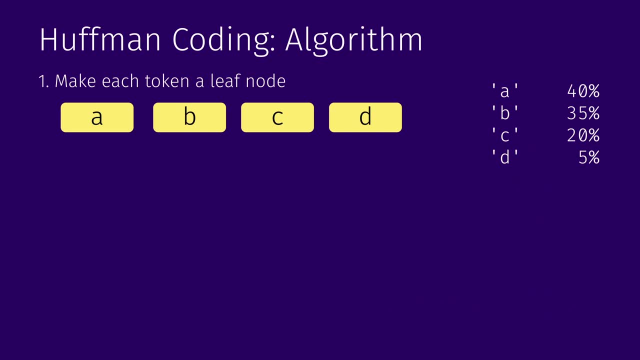 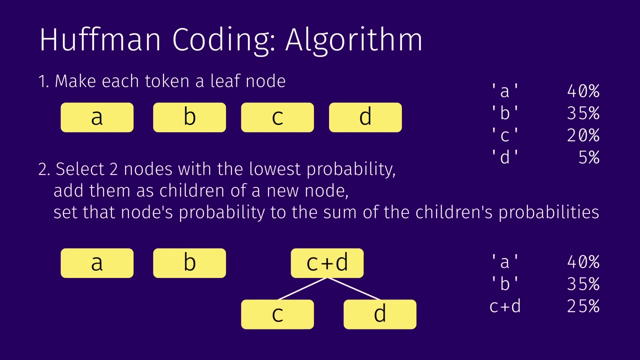 tokens and that what you will actually use for encoding and decoding. but you can only get those maps if you build the tree first. so how do we do that? first we make each token a leaf node. then we continuously repeat the following step: we select two nodes with the lowest probability, add them as children of a new intermediary node, set that node's. 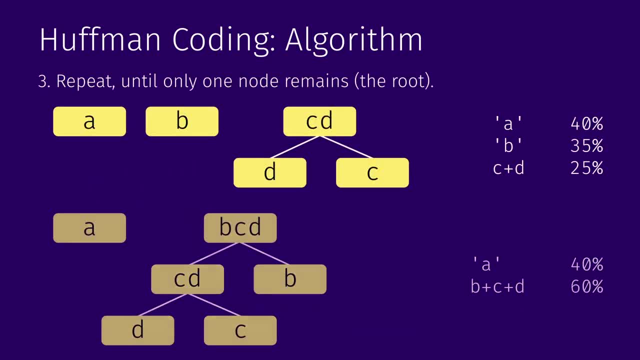 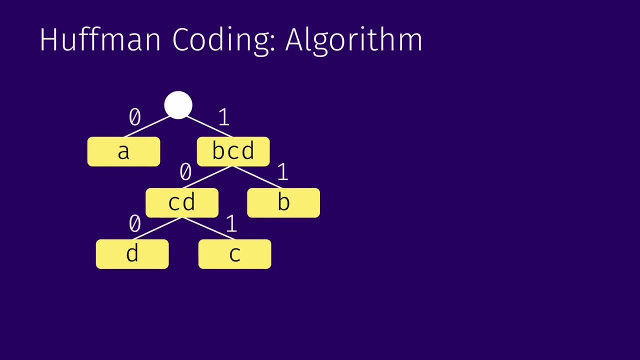 probability to the sum of the children's probabilities. we repeat this step until we only have one node remaining, and this node naturally will be the root of our tree. then we will use for encoding, we will start from the root and we will walk the tree recording the prefixes. 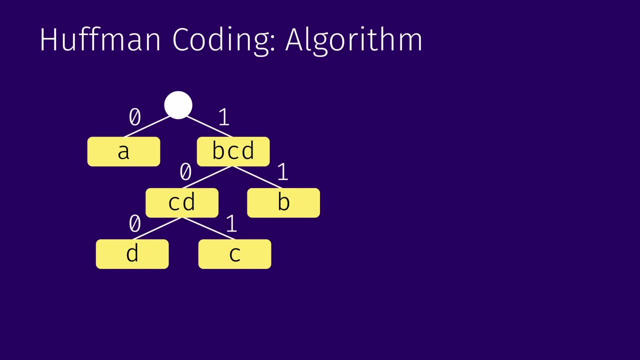 of each leaf. so, for example, if we go first right, taking one to b, c, d, and then we go left to c, d and then we go left again to d, we get one zero. zero and this is our prefix code naturally turns to the left. by convention are the same as zero and 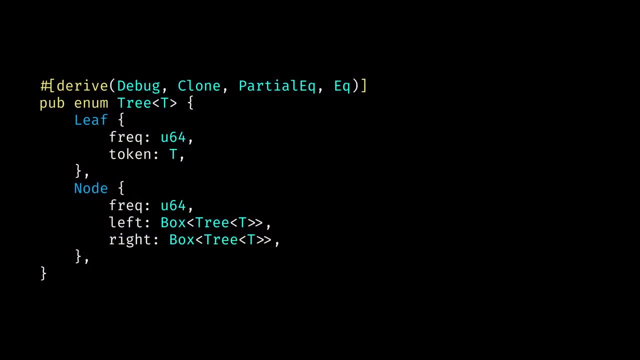 to the right are the same as 1.. And now we can start coding that in Rust. First of all, of course, we will need to start with the data structure for the tree. It will be an enumeration and we will have two variants in the tree. enum: Leave is a leave node with the token: The type of the token. 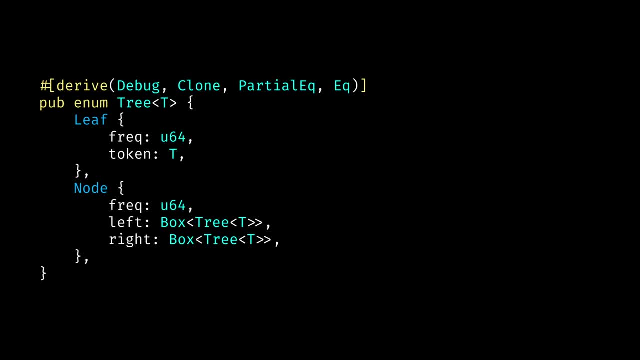 is generic, it's T, And we also store the frequency for this token. For simplicity, we will not try to normalize frequencies, So this will be just an unsigned integer. Second variant: in the tree, enum is node. Node will also have frequency because, remember, we need to sum frequencies of the. 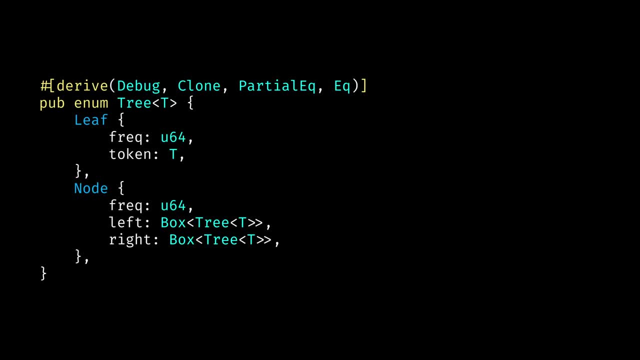 children to build nodes And the node will have left and right children. Now let's look how a little snippet of our example tree will be represented in this case. for convenience and for us to be able to write tests, I also did several accessor methods- Pretty much all those. 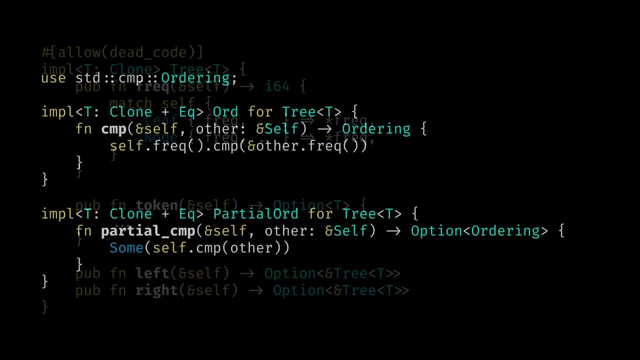 functions look the same. So let's start with the example tree And we will have a little snippet like the frequency function you can see here. To efficiently select the lowest probabilities nodes we will need to use a heap. Rust's standard library already provides a binary heap. 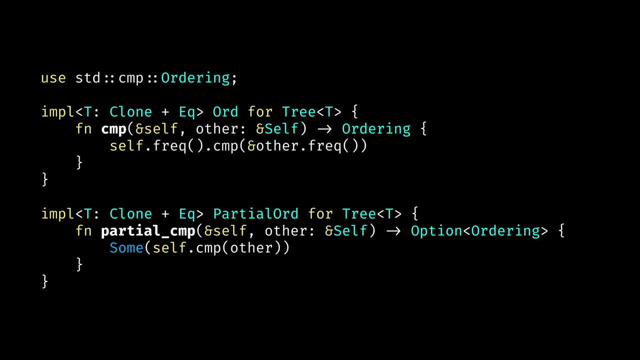 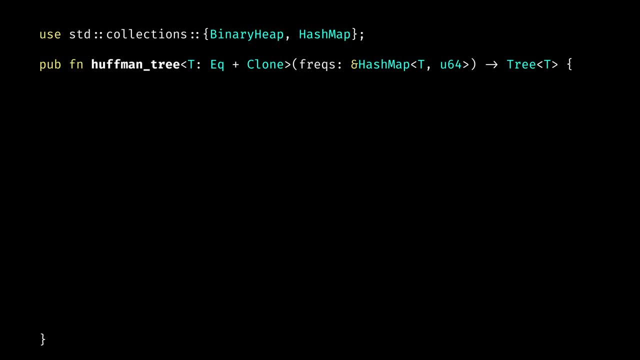 So you need to be able to compare nodes between each other. So we will need to implement ordering and partial ordering for our tree type Binary heap that Rust implements in the standard library by default will allow you to select the maximum nodes, And we need to select. 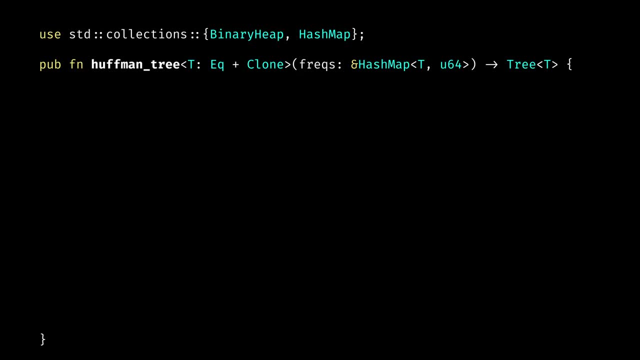 the minimum nodes. But thankfully Rust standard library also provides us with a handy data structure called reverse that you can use to wrap whatever you have to reverse ordering. So if, instead of adding our leafs and nodes to binary heap without reverse, we will add them with reverse, it will mean that our binary heap will work as a min heap. 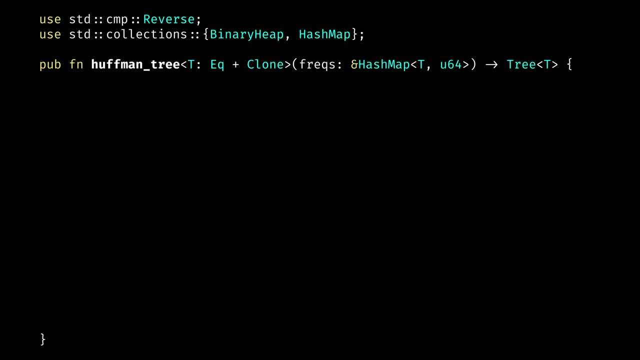 which is what we need here. Let's look at the core algorithm Now. we implement this function. we accept the type of tokens as a generic parameter and we take a frequencies map for our tokens. We create an empty heap and we put all of those tokens as leaves in this heap, using reverse to. 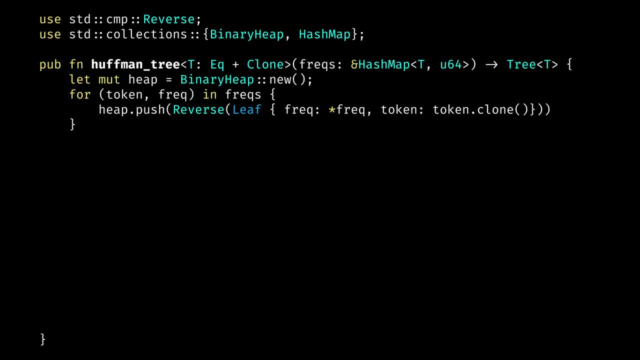 make sure that we will first fetch the least frequent tokens from the heap and then, as long as we have more than one element remaining in the heap, we will select two nodes with the lowest frequency from the heap. We create a merge node where we will add frequencies of the children. 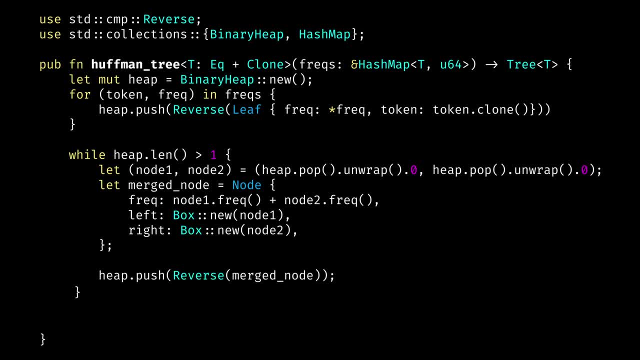 together and we will set those nodes that are selected as left and right children of the merge node. Then we will push it back into the heap. In the end, after we only have the root node remaining in the heap, we pop it out of the heap. 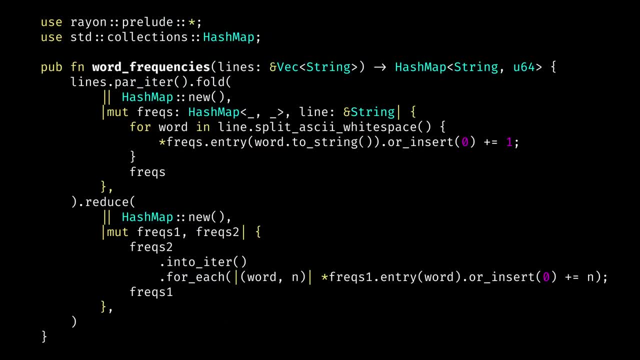 we return it Now. I mentioned that we will need to get frequencies of the tokens to actually build the tree, so here you can see an example how we can do it and how we can do it in parallel as well. Here we accept lines, which is a: 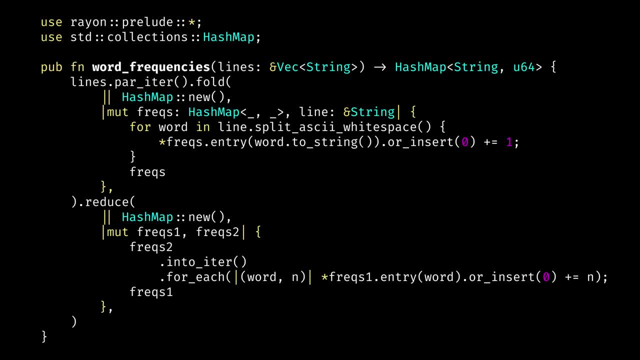 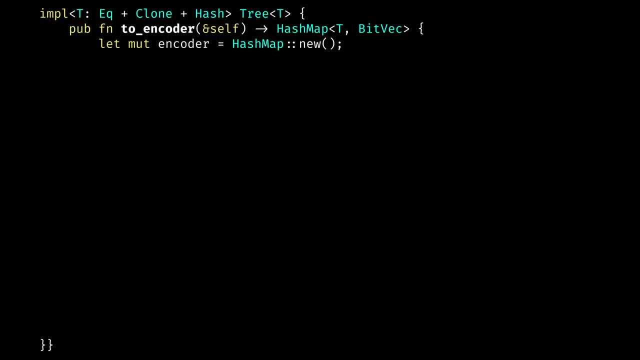 vector of strings and we calculate word frequency in this case. so each token is word. so we will return a hash map from strings to U64.. Naturally you can implement similar methods for all kinds of tokens. they don't said need to be strings. Now we can finally create an encoder. This is a hash map from tokens. 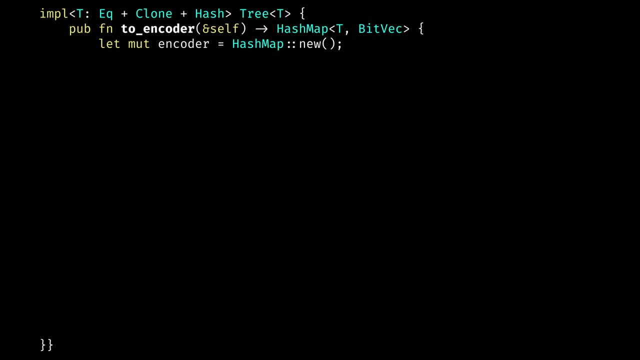 to Bitvac Create, named bitvac as well, and it allows you to efficiently store vectors of bits- and in our case our encoding works on the level of bits, so you need to be able to somehow store them direct. you can, of course, express them as your aids, but then you probably will not. 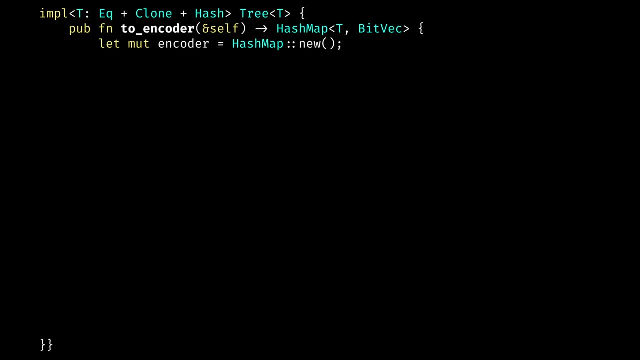 achieve that you for any compression, because you will waste a lot of space. Bitvex solves this problem. It allows you to work with a collection of individual bits pretty much the same way as you would work with a normal vector. To create this hash map, we will need to work the tree that we generated. 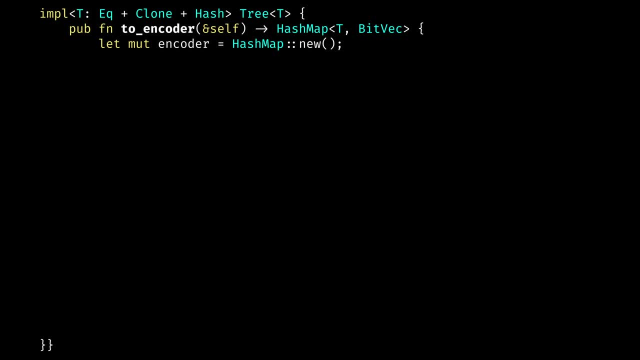 And to work a tree, you have two broad choices. Normally, you can either use recursion or you can use stack, And we will use stack first. We will start with putting the root node together with an empty bitvector. We will use bitvectors to, of course, trace the path to each. 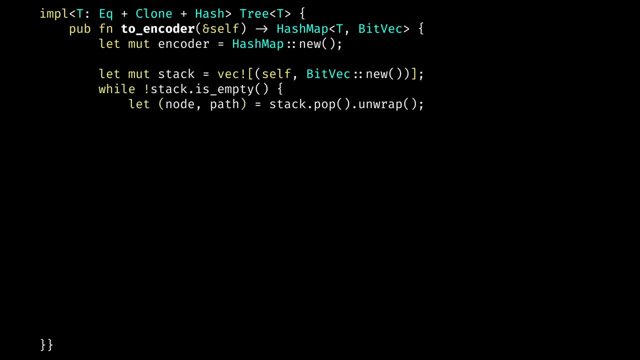 node on our stack And then, as long as the stack is not empty, as long, in other words, as long as we have more stuff to explore in the tree, we pop the first element from the stack. we create variables, node and path from that popped element and we might. 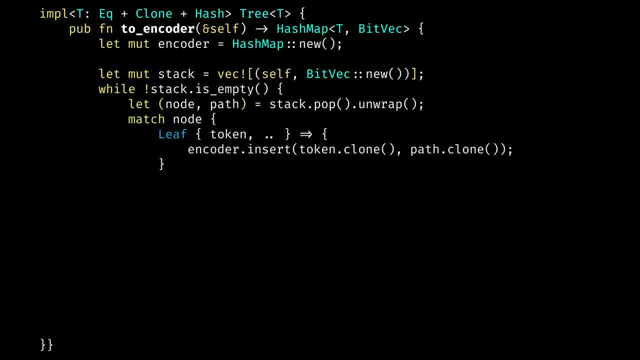 run a hash node. If it's a leaf, then we know that we found some token and we now should have a full path to this token. so we insert this token as a key and this pass as a value in the encoder map. If we encounter an intermediary node, then we know that we need to walk both left and right. 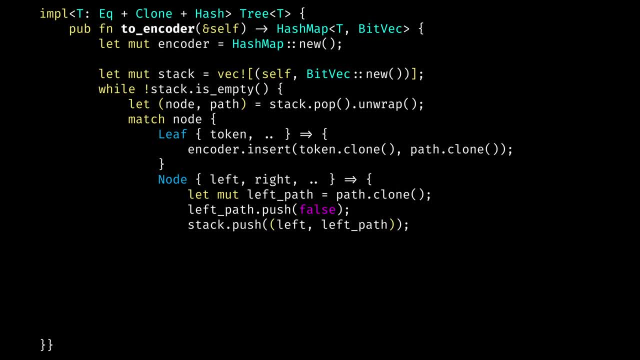 children, For example for the left child, we copy our path. We add one zero bit. Here we need to write for a chunk of the network, So we add one zero bit. Now we have to be careful with the number of nodes and array And if there are no nodes left and right, then we are only working with 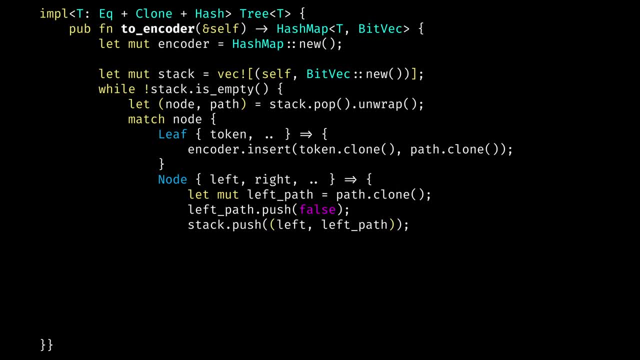 the number of nodes. So we have to be careful with the number of nodes and array. And if you have, that's the API of the bitwag, but think about it as zero- We add it to the path and then we push the left child together with this left path on the stack And we do the same thing for the right. 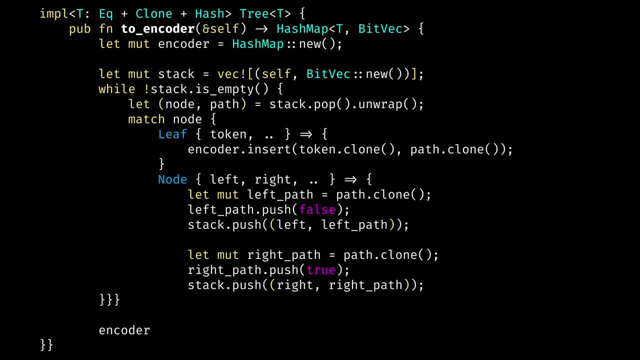 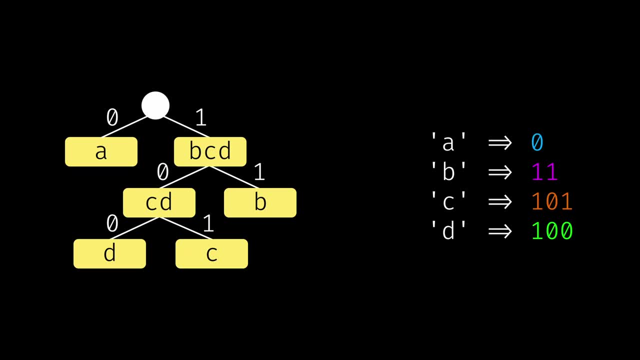 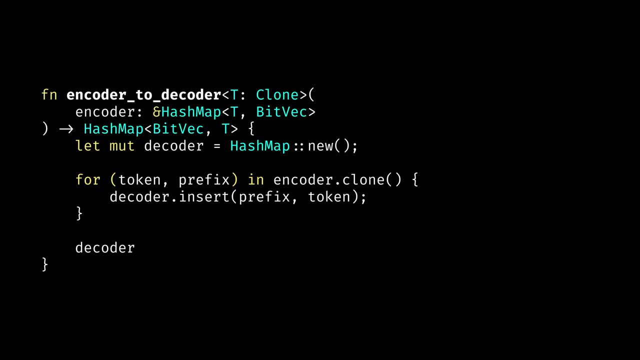 path And in the end, once we finished working the tree, we return the resulting encoder hashmap Function. to encoder will essentially take us from the tree on the left to the hashmap on the right, And to decode whatever we compressed back in a readable format, we will need to essentially. 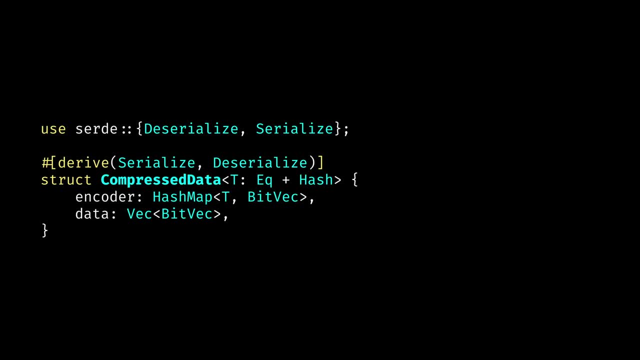 reverse the hashmap. Now we need to figure out how we will actually serialize our data structure. So far, everything has all happened in memory, but we of course would want to write something to disk. We will just use Cerda. I will be using message pack with the beautiful RMP library that. 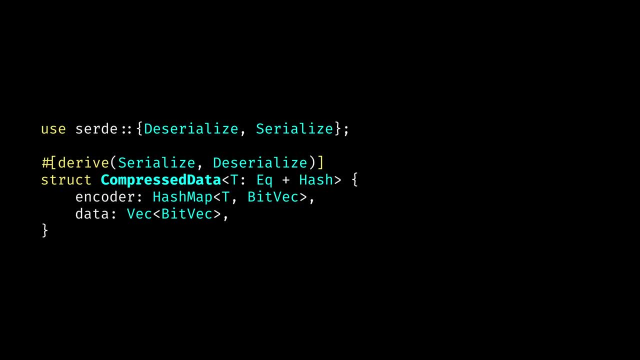 provides message pack encoding. In any case, the particular encoding format here is not that relevant. You can select something else, for example bin code, As long as it doesn't add too much overhead, we still should achieve compression. Of course we will need to write. 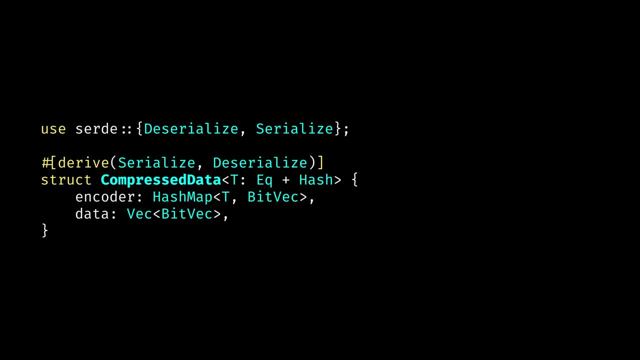 our lines. We will represent them as vector of bitwags, each line encoded using our Huffman coding, And we also need to remember which tokens were mapped to each vector. So we also add in encoder hashmap from tokens to bitwag. Of course you can use decoder hashmap here instead. 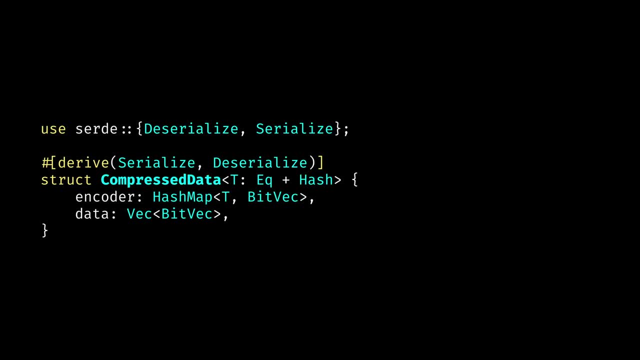 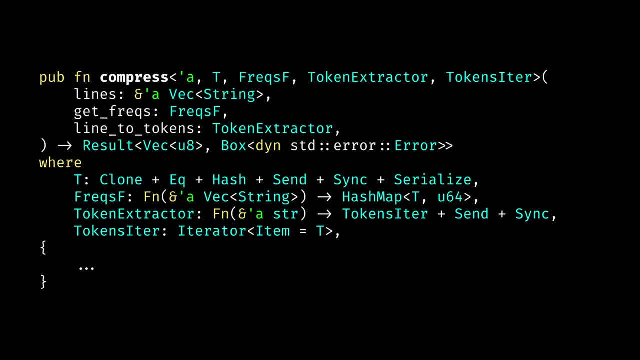 which will mean that the coding will be a bit faster, but encoding will be a bit slower because you will need to transform your hashmap. And now we are ready to write our compress function. I wanted to try two approaches with this algorithm. I wanted to try to encode our file using words. 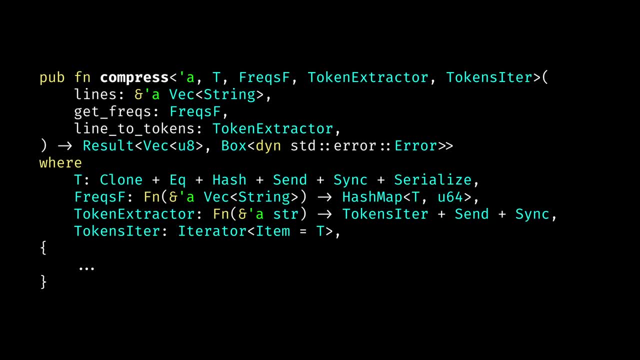 individual words as tokens And I wanted to try encoding stuff using individual characters as tokens. We will need to accept two closures, And that makes the signature of that function somewhat similar. So we will need to accept two closures And that makes the signature of that. 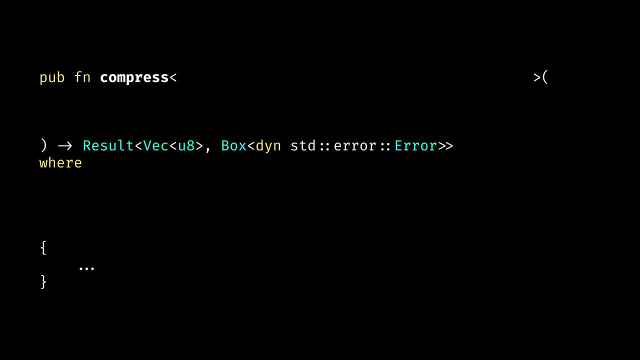 scary, But let's take it step by step. And, of course, remember I did not come up with this signature from the top of my head. In fact, I was just allowed compiler to guide me to write it, And whenever you write something like that, compiler will tell you: oh, you forgot this. 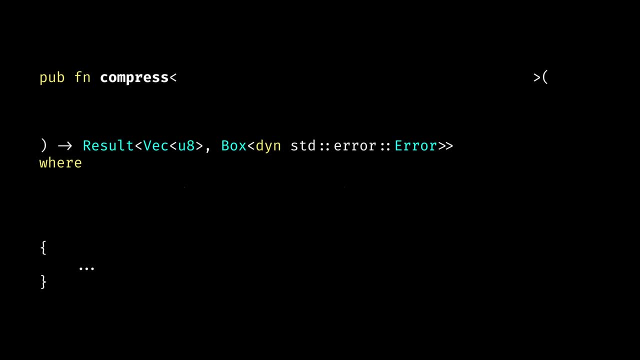 trade bound here, or you need to add lifetime parameter there. As long as you follow its instructions, you usually will be able to write such signatures without much thought. In any case, we will start with a reference to our lines vector, And then we have two closures: get frequencies and line to tokens. 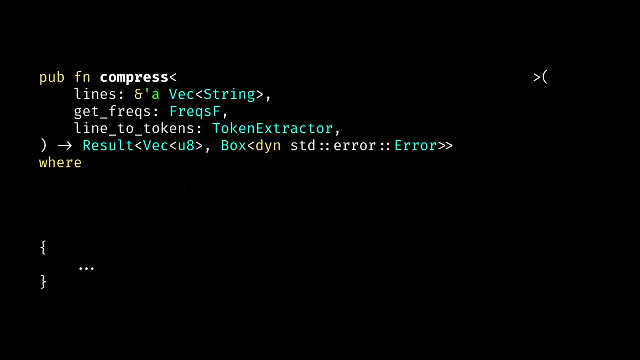 Get frequencies is responsible for extracting frequencies from lines. For example, like the word frequencies functions that we saw before, Line to tokens is a function that allows us to split individual lines to tokens. Whole compress function will return a result And, in case we 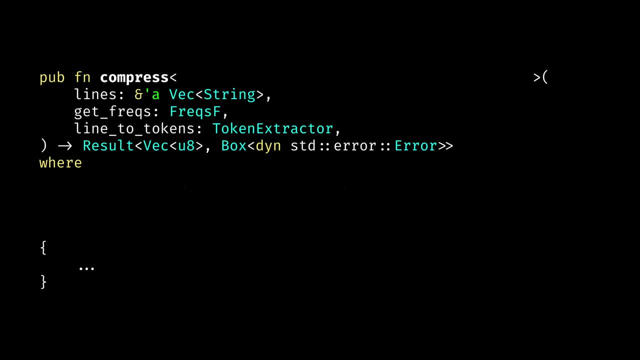 succeeded, we will get a vector of byline, And then we have two closures And then we have two combien to ones, So we can find the full line to token in the linear descent, And then we will have a string that supplies something that we can then write to a file or send over a network. 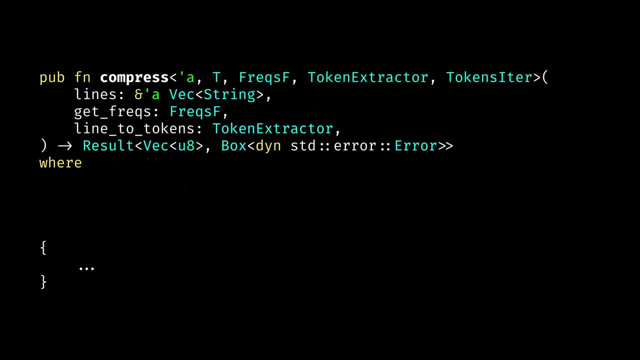 We need to provide trade bounds for all of those generic parameters, And now we have quite a few of them. We have C for our token type. we have frequencies F for our get frequencies closure. we get token extractor for line to tokens closure. We also need to introduce lifetime. This is the 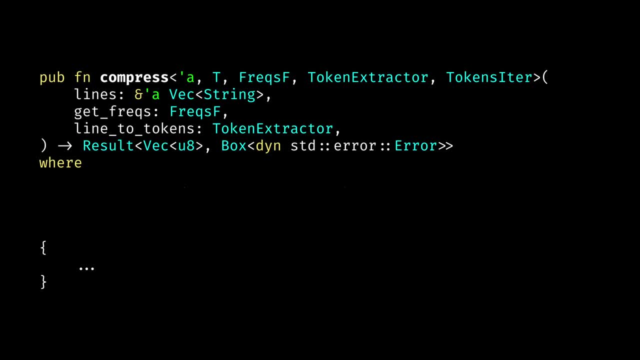 requirement here because we have too many references and compiler needs a bit of our help figuring out how long each of those lives. And so. To get least of the five, we need to wear a � The tokens need to be cloned, they need to be able to be compared, they should be able 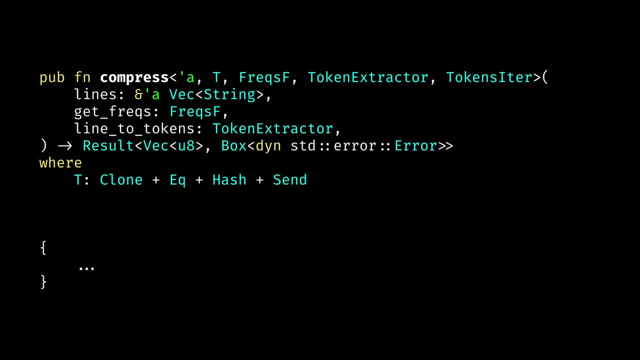 to be stored as keys in a HashMap. they also should be thread safe. we will also use rayon here to speed up our compression a bit. we also will need to be able to serialize our tokens For our frequencies. closure: just accept a mutable reference to line and we return a. 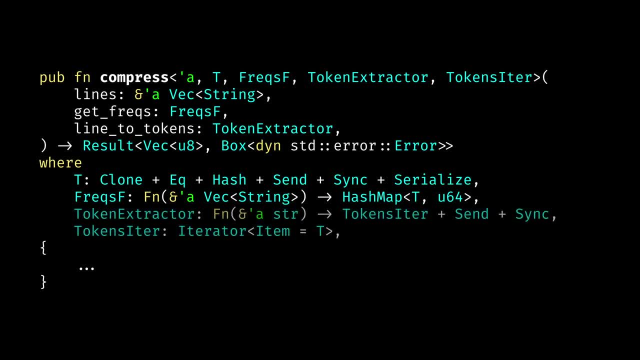 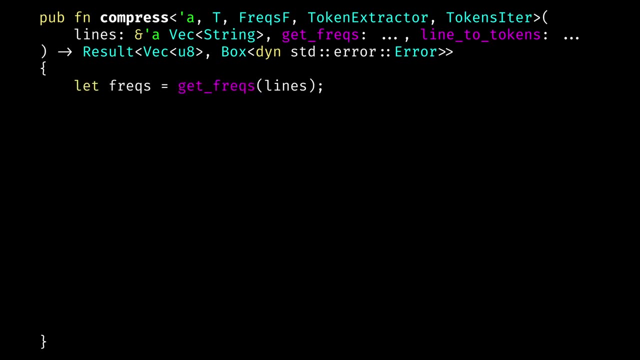 HashMap of frequency of the tokens. Then extractor takes reference to a string and returns an iterator over tokens that also should be thread safe. Now the body of this function is way simpler than its signature. First, we get frequencies of our tokens by calling the getFrequencies closure on our 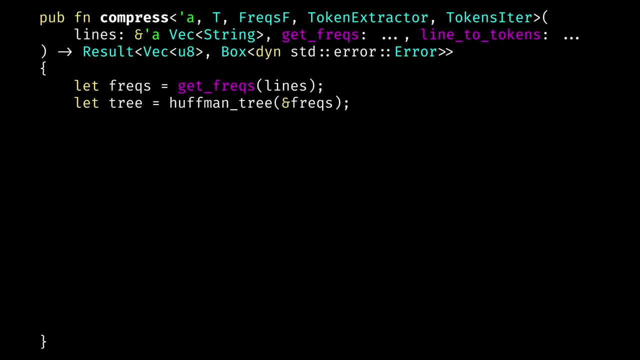 lines. then we call our Huffman tree function on the reference of frequencies to build the Huffman tree. then we convert it to a HashMap with toEncoder function And then finish the code For each line using parallel iterator we map to its binary encoding. for that we split. 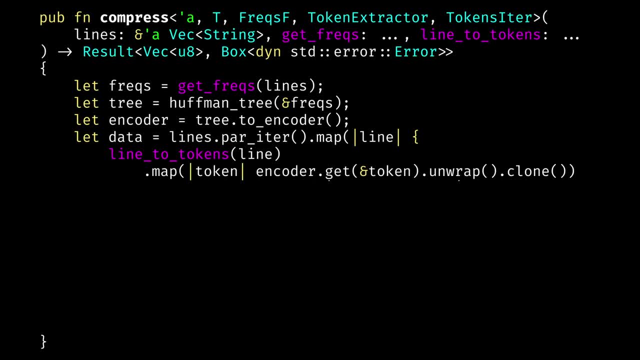 line and tokens using line to tokens closure- then we map each token to its encoded version, which will be a bit vector, and then we join all those bit vectors together. In the end, we collect all of that into a vector. Now we create the compressed data structure which contains our encoder and our data, and 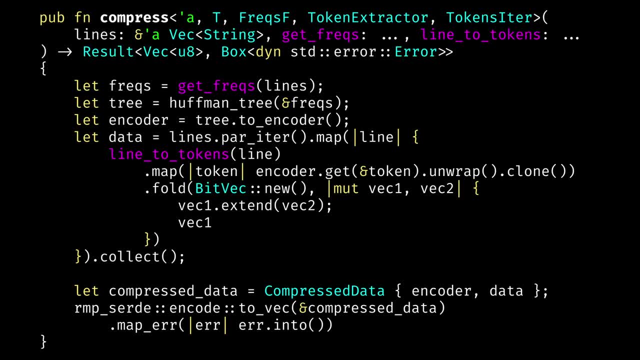 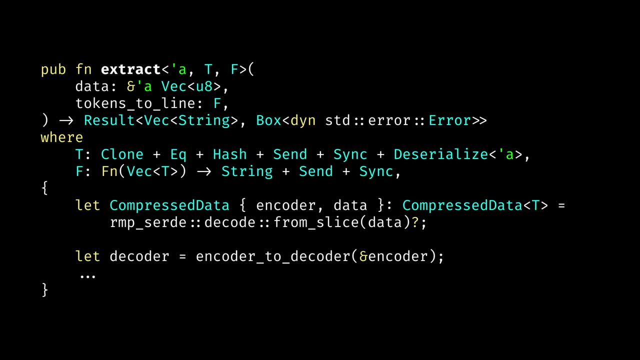 we use RMP server to convert it to the encoder. Now we can compress the data, but how do we extract the data? We only expect to get a reference to a vector of bytes as our data, and we also accept a closure which is called tokensToLine, because now we need to do the reverse transformation. 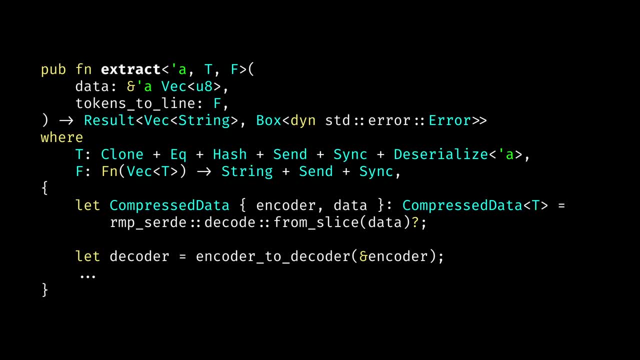 we need to take tokens and we need to somehow merge them to be one line And this function will return a result and if everything goes well, this result will be an OK of vector of strings, which is our lines. Now we just use RMP server library to decode our bytes, to compress data struct. 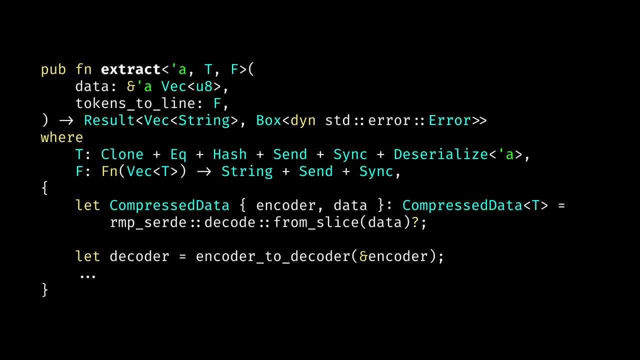 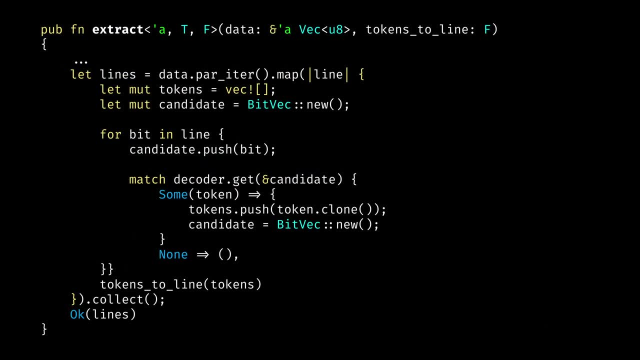 Then we call our encoderToDecoder function to convert our encoder that we stored in the file to a decoder hash map that we can use to extract tokens from the prefix code. And then we again use rayon, parallelize our execution. We convert our data vector to parallel iterator and for each of those lines we create a new. 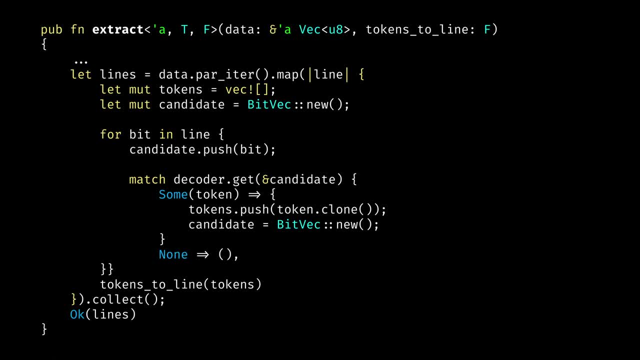 vector to decode And then we essentially try to match our token, progressively, reading bit by bit from the line. We push each bit into a candidate bit vector and then we check if this candidate is contained in the decoder hash map. It means that we read a token and we can push it into our token's vector. 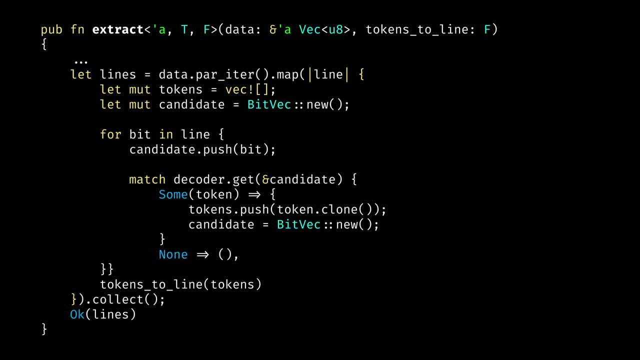 Remember, Huffman's coding provides us with prefix codes, Which means no coding. No code will be a prefix of another code. So whenever we found a match in the decoder struct, we know that we found a token. We don't need to care about storing lengths. 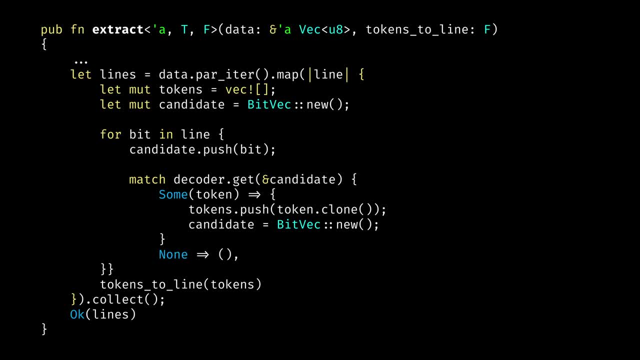 And we, of course, after pushing the new token, we need to drop all the stuff from our candidate, because now we start to read the next prefix And if we didn't get a match from the decoder then we just don't do anything. 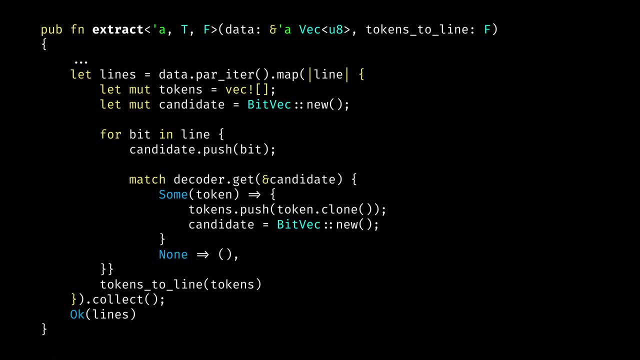 After reading all the bits in the line, we convert this to the actual string By using tokens to line closure, calling it on the vector of tokens, And, of course, to compute all the lines we collect and we return it as OK lines. 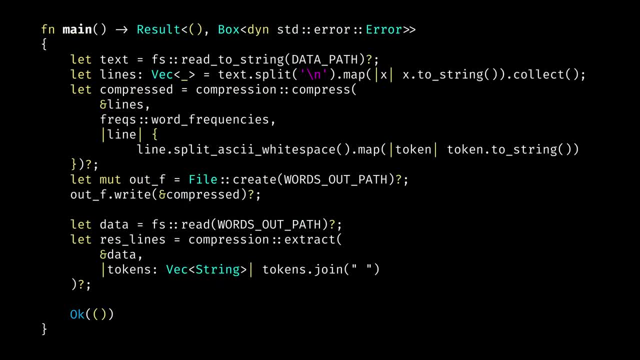 And now we are done. This is a very simplified version of our main function. You can check the repositories that I will link with the actual implementation, because it uses club to provide some command line arguments and niceties, like tracking time, for example, for each step. 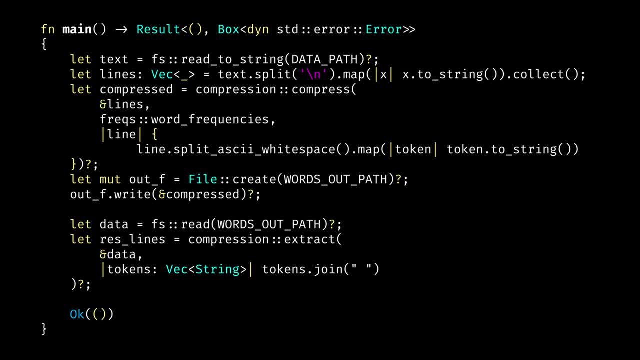 But On a very high level. we read our file to a string, we split it into lines, we then call our compress function. we then create a file for our compressed representation where we write compressed data And to decompress, we read the compressed data file and we just call our extract function. 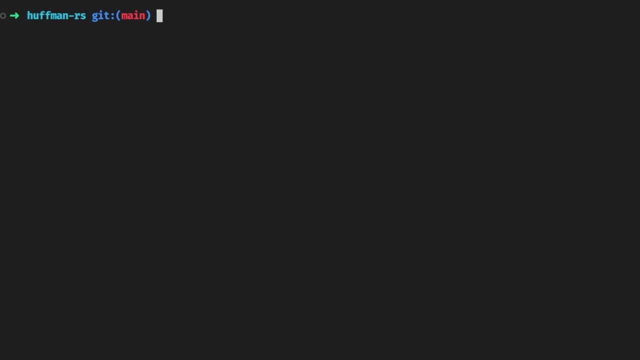 passing the closure for joining our tokens into it, So let's run it. We will be using a Wikipedia dump- English Wikipedia dump- For this example. you can find instructions. You can get this data in the repository as well. It's just from Kaggle, one of the open data sets. 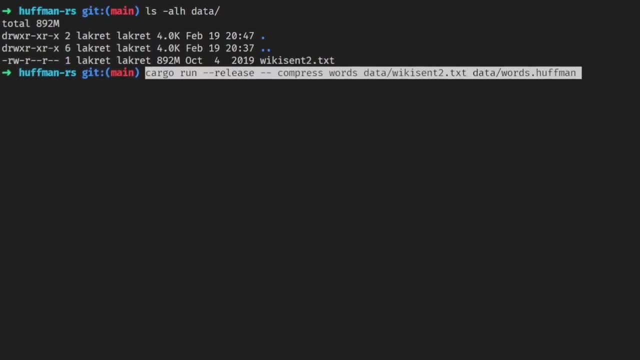 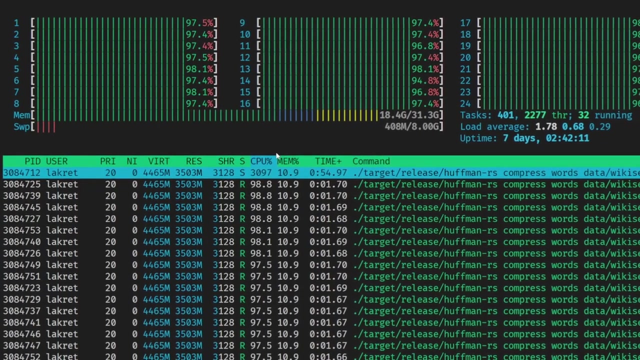 It's about 900 megabytes large. You can see that our interface has compressed and extract arguments and we can select between words and chairs. We can see that we are using our course very efficiently when we run it. We can now see that. 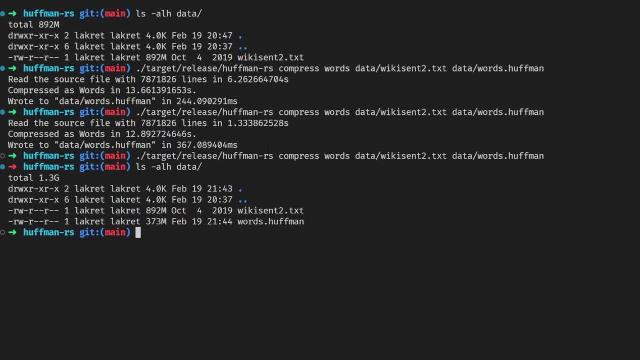 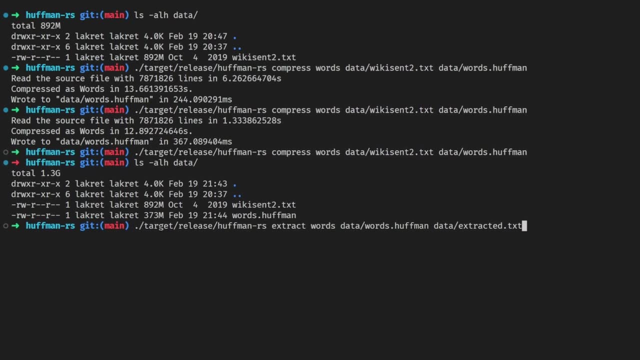 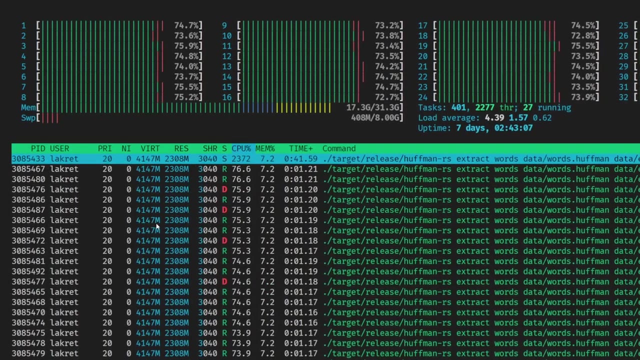 Our, Our compression was successful because instead of almost 900 megabytes we arrived at 373 megabytes. Of course we can use the same utility to extract, And again we can see that Rayon helped us speed up some stuff. 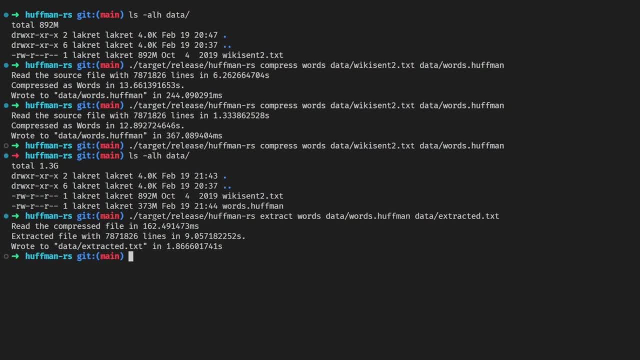 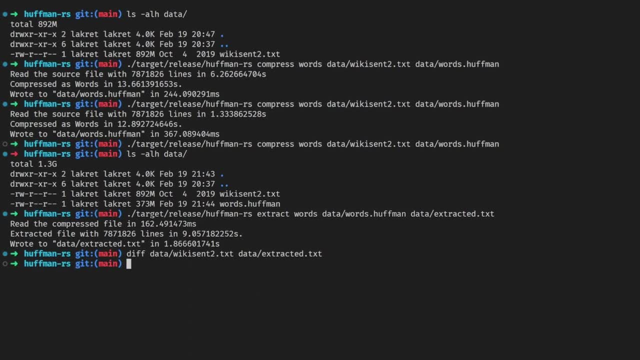 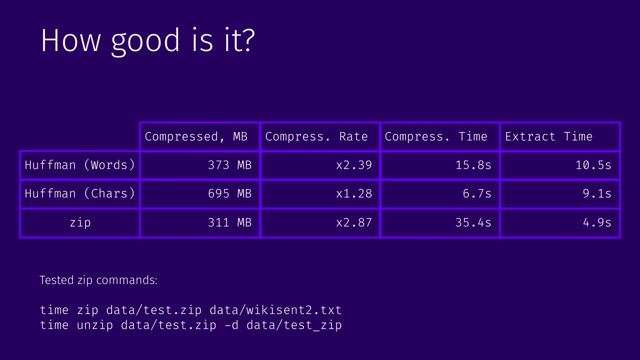 Now to verify that our compression doesn't lose any data, we can run div on those files And you can see that nothing is returned from the div. We can be sure that our files are identical. Apart from that, I also looked at using Chars mode and I also compared it with Zip using 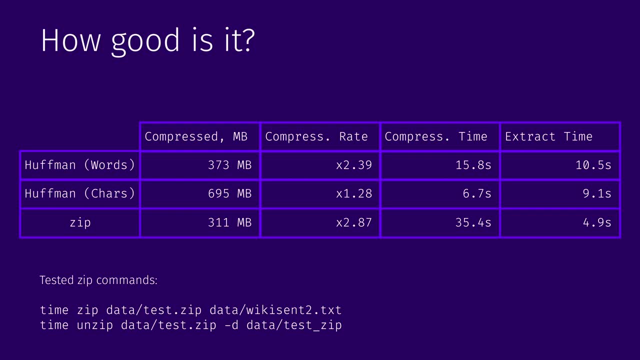 standard settings without any modifications And surprisingly enough our compression rate is quite close when we use the words mode. But of course our algorithm is very, very basic and not production ready. We haven't put much thought yet into optimizing it. Compression time in our case is also faster because it seems that by default Zip doesn't 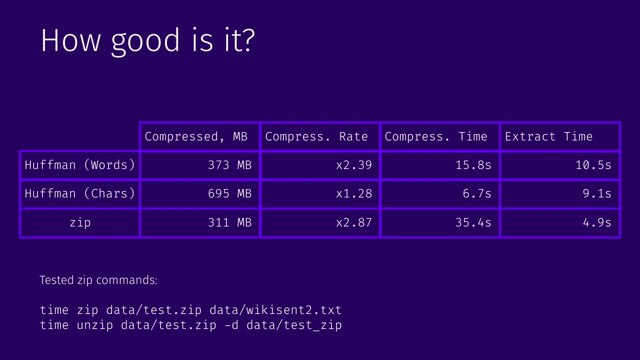 try to scale across multiple cores. However, Zip outperforms us on extraction time. If you look at Chars encoding, you can see that we don't achieve nearly as good compression rate, even though our compression time is very, very fast and our extraction time is. 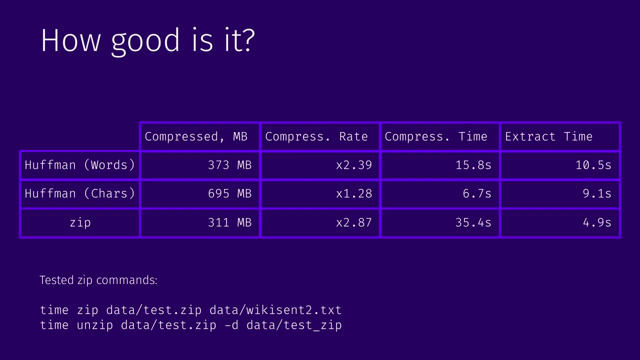 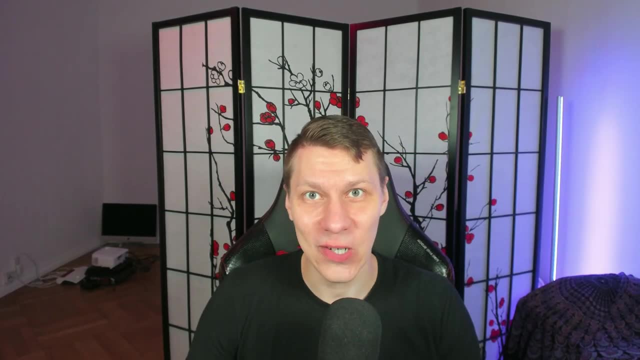 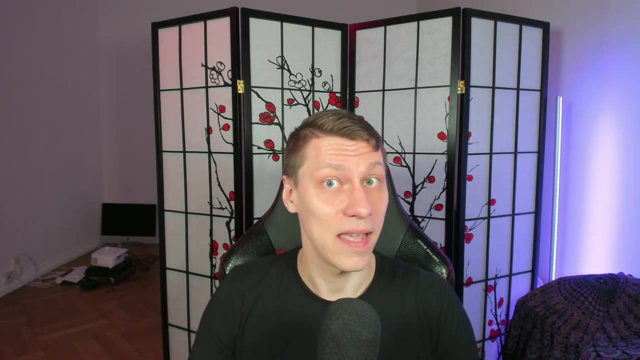 also quite fast. So you can see that, depending on the choice of your tokens, you can achieve different compression. So thank you for watching. Please don't forget to like and subscribe, and if you have any questions, don't hesitate to write a comment. 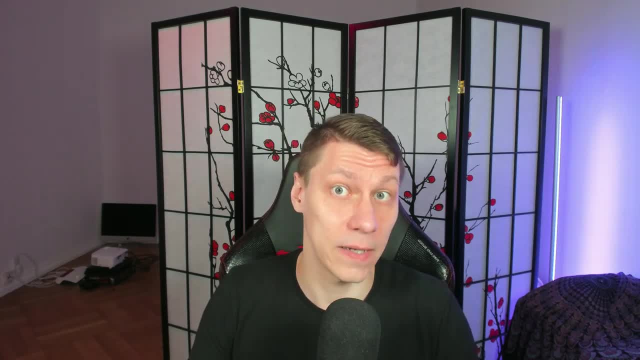 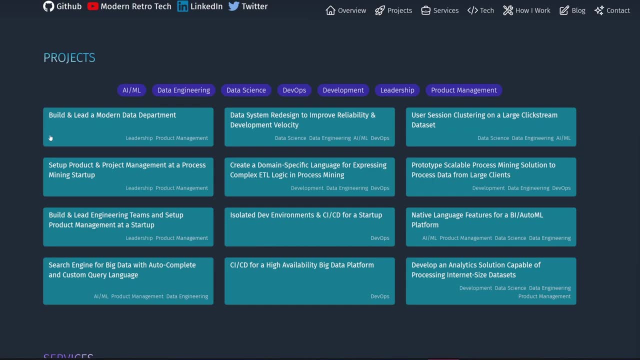 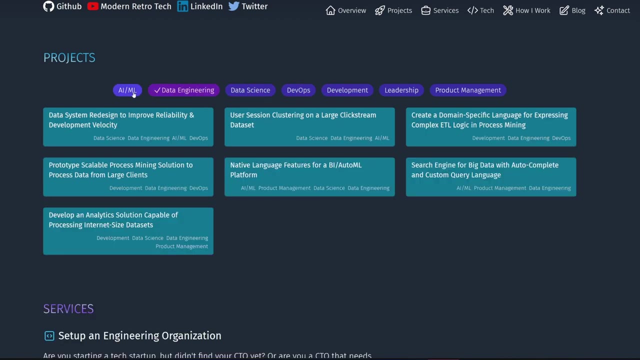 And I have a bit of news. Recently I started providing consulting services and I have a new website, so please don't hesitate to check it out. I also have a blog there, which I will try to update from time to time And, of course, if you or the company you work for requires consulting services for anything, 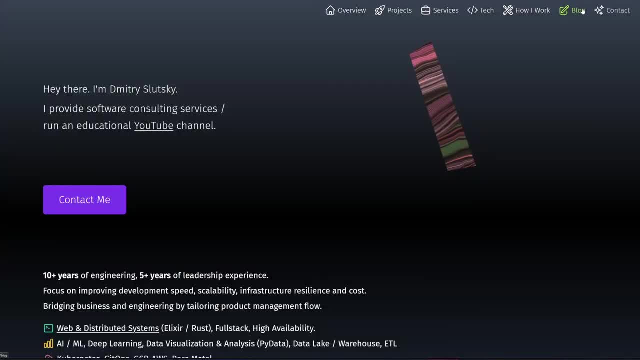 related to Rust, Elixir, web development, distributed programming or data stuff. there is a contact form on the website through which you can easily reach me.